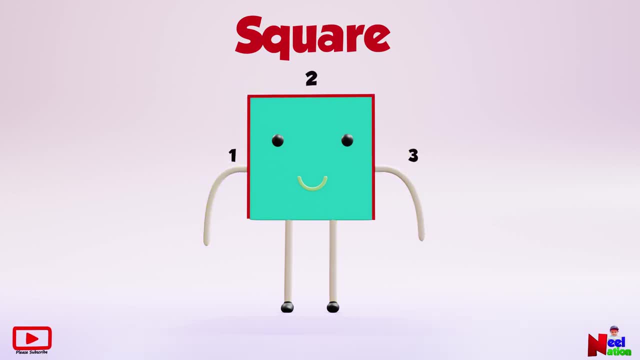 two, three, four, Four sides And one, two, three, four, Four corners. Bye bye, Bye bye. Hello, there, I am a triangle. I have one, two, three, four, Three sides And one, two. 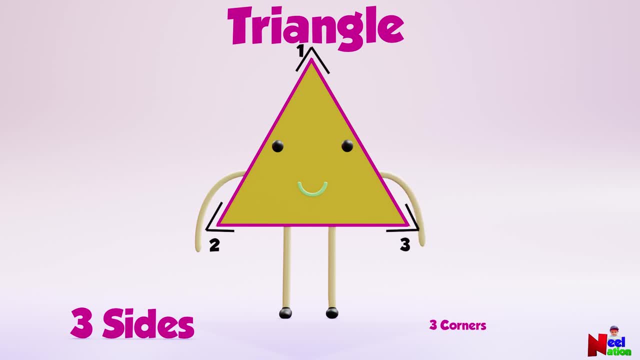 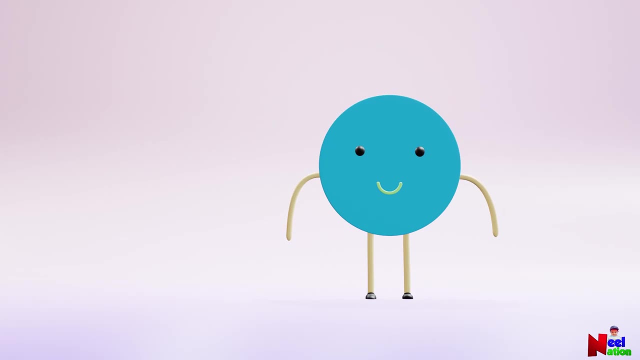 three, four, Three corners. See you later. Hello boys and girls, I am a circle. I have one, two, three, four, Four sides And one, two, three, four, Three corners. Here is my word. I don't have any corners, Zero corners. 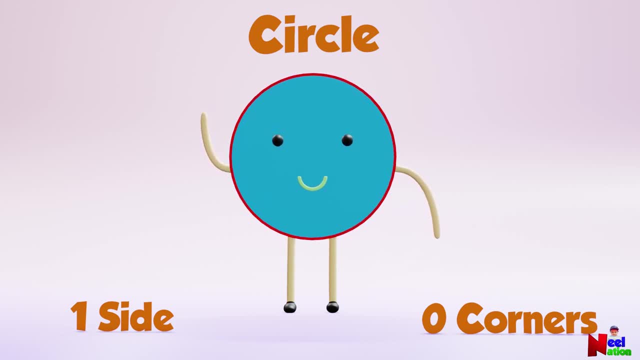 Bye, bye, Hello, Hello, boys and girls. I have three corners. I have one, two, three, four, Four sides And one, two, three, four, Three corners. One, two, three, four, Three corners. Hello, Hi, I am a circle, I am a triangle. I have one, two, three, four, Three sides. I am a triangle, I am a rectangle. Here you go, Ten corners. I have a circle, I have one. 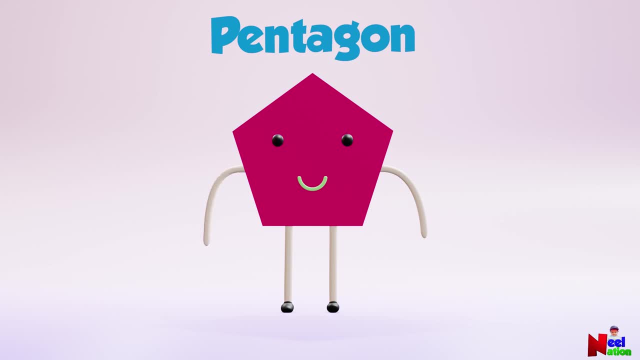 I have one, two, three, four, five, five sides and one, two, three, four, five, five corners. Bye-bye, Hello, there, I am a second. I have one, two, three, four, five. 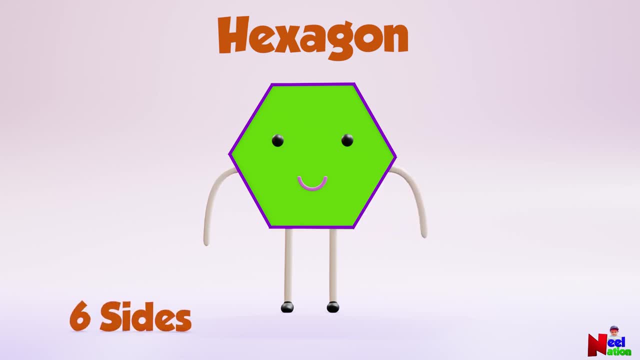 I have one, two, three, four, five, six, six sides and one, two, three, four, five, six, six corners. Bye-bye, Hi, I am an oval, I have one third side. I don't have any corners. 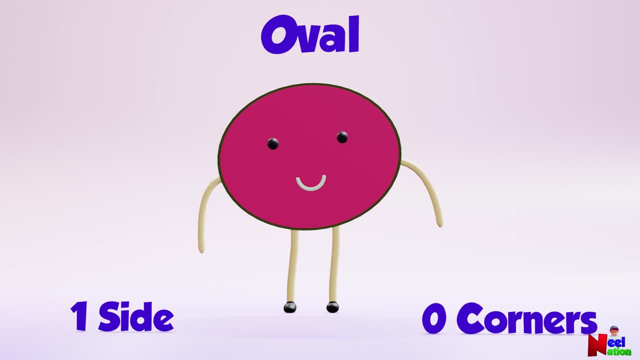 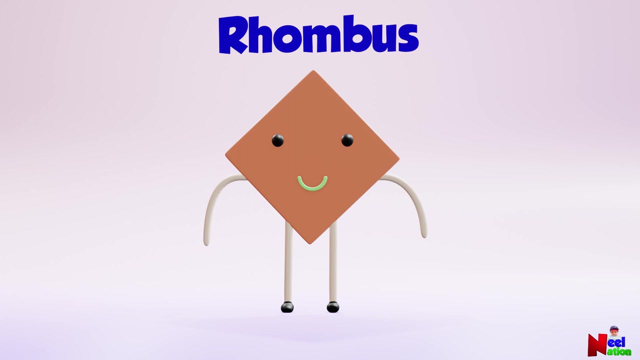 Zero corners? No, no, no, Bye-bye, Bye-bye, Bye-bye, Bye-bye. Hello, I am a robot. I have one, two, three, four, four sides and one, two, three, four corners.